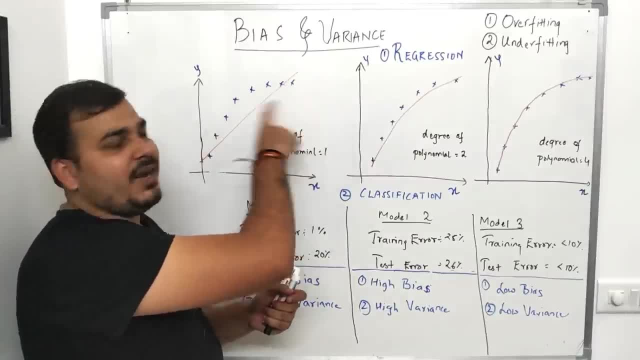 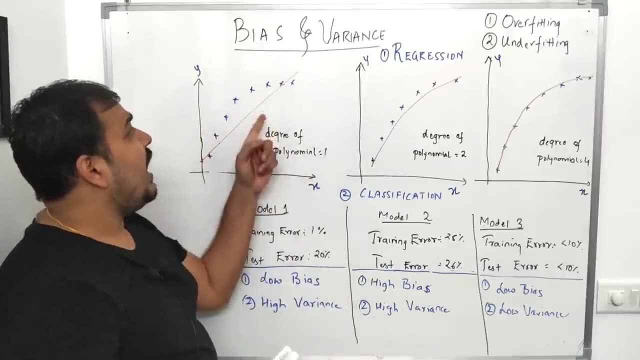 here my point is actually spread in this particular shape. right, It is in this particular shape. So in the shape of a curve. but if I have degree of polynomial is equal to 1, I just get a best fit line. Now when I compute the R squared error, definitely the R squared error will be high, You know it will. 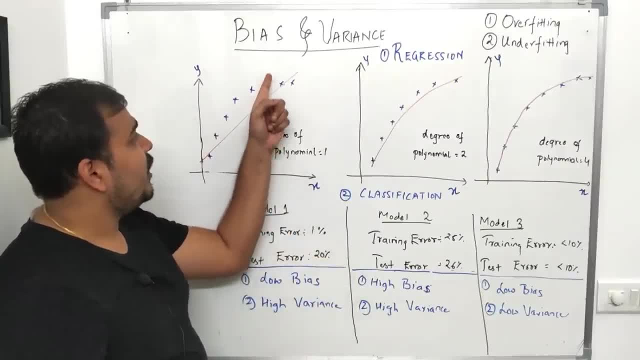 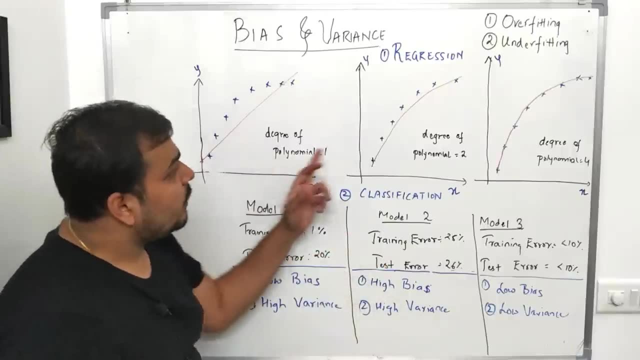 be on the higher side because, again, you understand, this is my predicted point, This is my actual point. If I do the summation of all the errors right, it will be usually high. right Now, suppose if I increase the degree of polynomial is equal to 2 in the polynomial linear regression, what will? 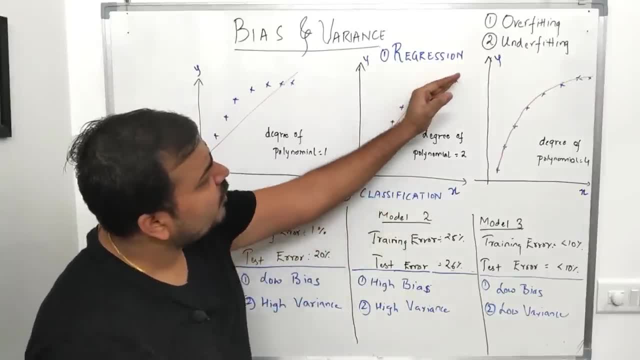 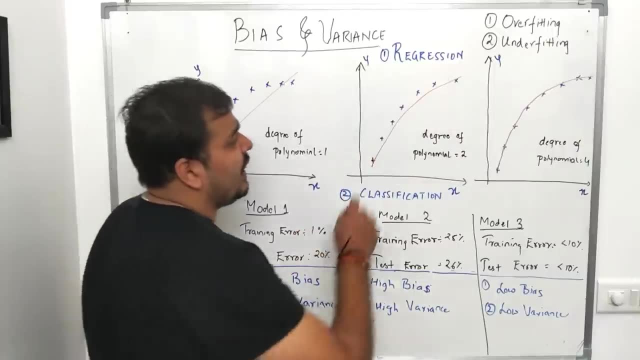 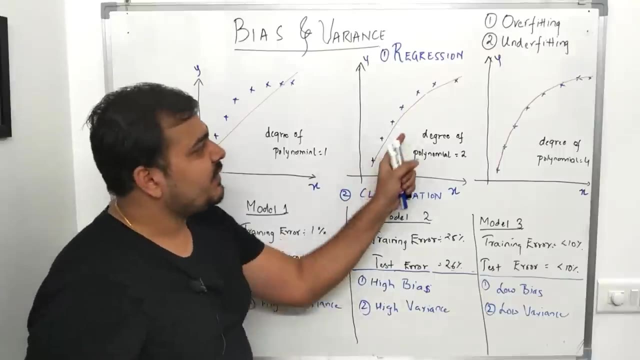 happen is that now the best fit line will actually become a little bit smaller curve. right, It will be a little bit smaller curve. Now, in this scenario, you can see that it is actually satisfying most of the training points and definitely the error is very, very less right. The error is very, very less. 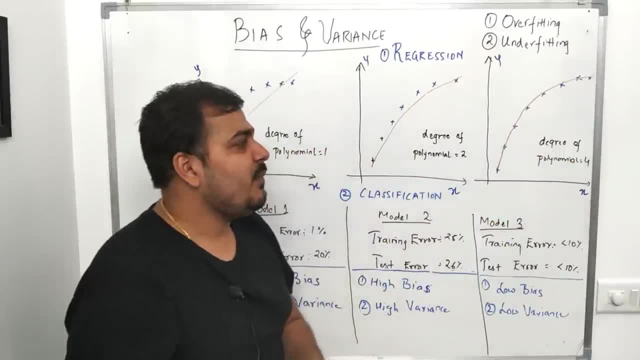 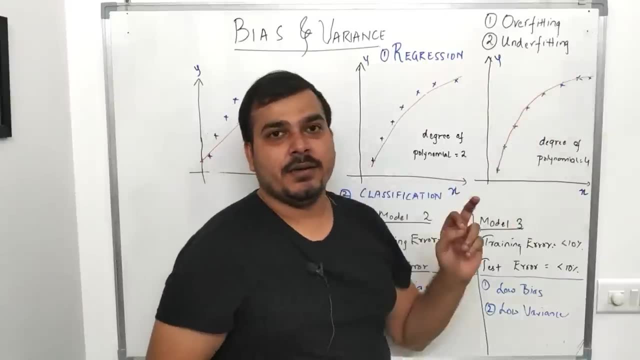 Now let us go one more step ahead. If I make, the degree of polynomial is equal to 4.. Now you can see that this is a condition where each and every point is exactly fitted to this particular curve line. Now let us go back ahead to this particular thing only When my error is very, very 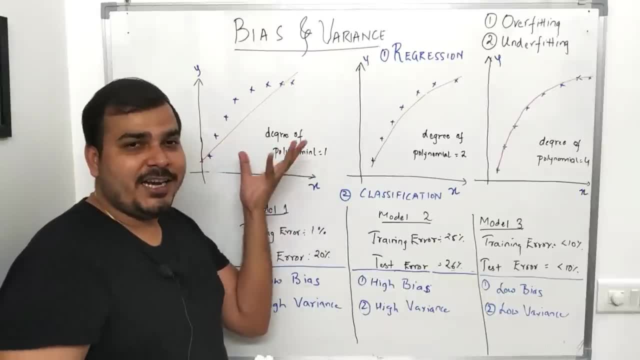 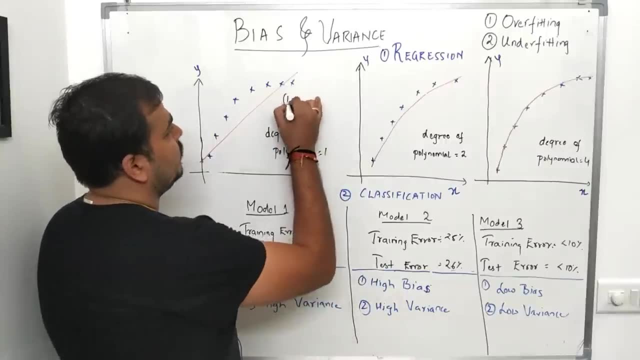 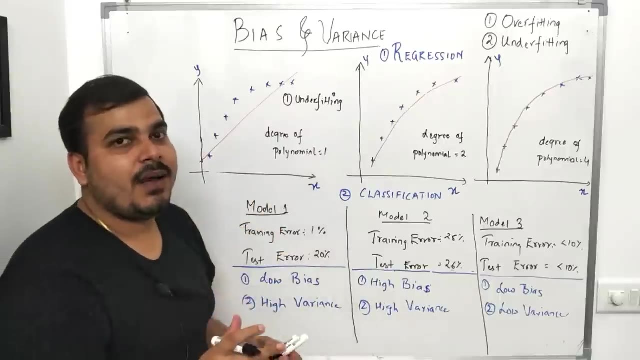 high and I understand that we have created a model on a training data set and for the training data set it is giving a very high error. So this scenario we basically call it as underfitting right. Underfitting basically says that for whatever data I have trained, my model, the error, 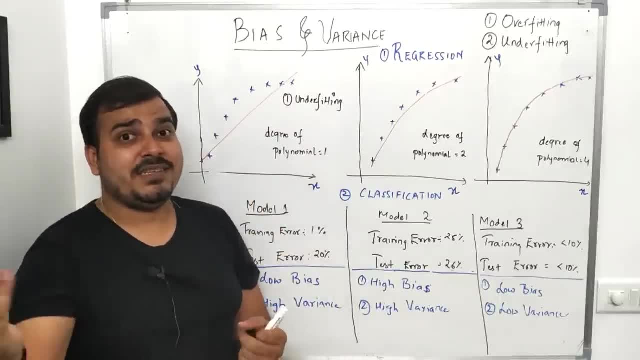 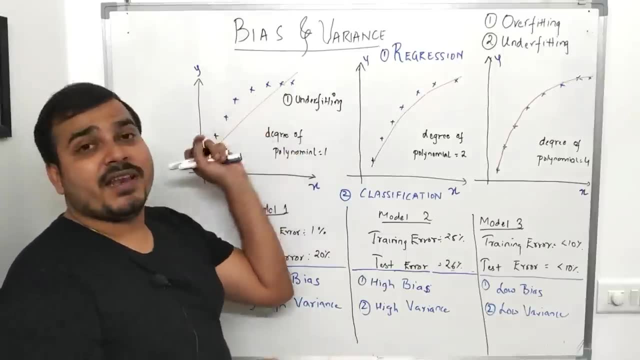 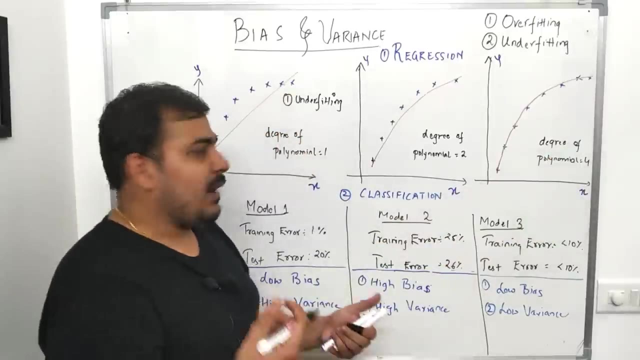 is quite high for that right. I'm just not talking about my test data or the new data. This is just only with respect to the training data. Even for the training data, my error is very, very high. So this is basically an underfitting condition. Now let us go back to the last diagram Over here. I 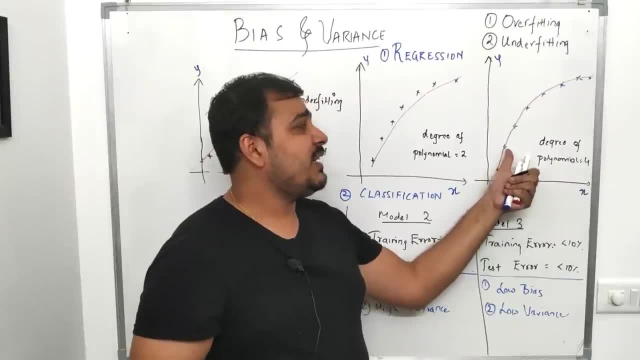 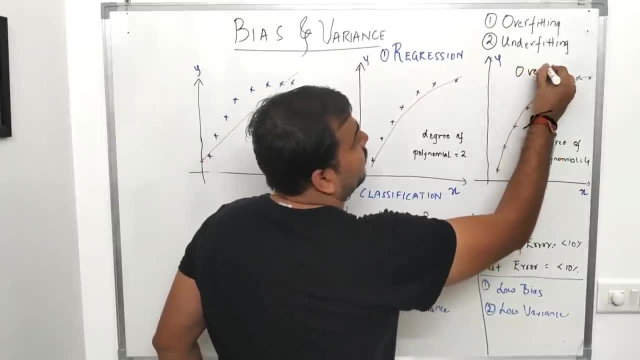 probably think you know about this now, since each and every point is getting satisfied by this best fit line right Now. this is a scenario where I can say it as overfitting. I'll tell you why we are saying it as overfitting. Now just understand, guys. OK, Now overfitting basically means what? 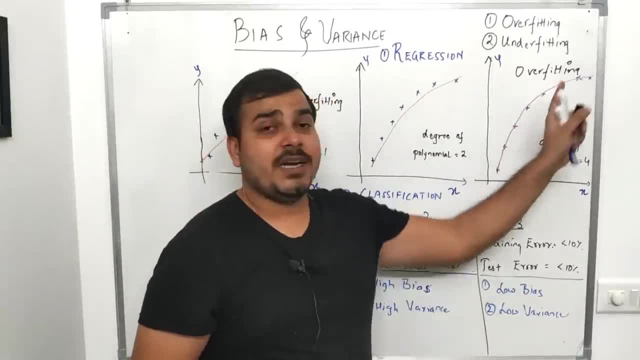 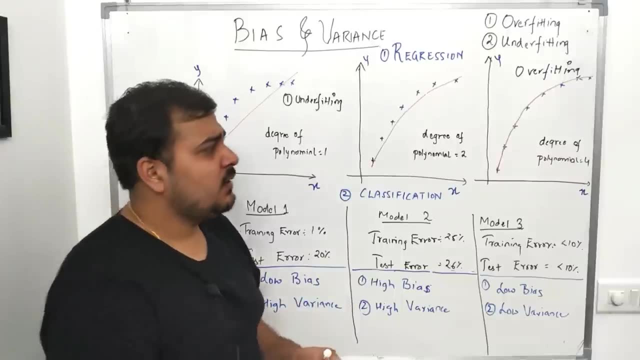 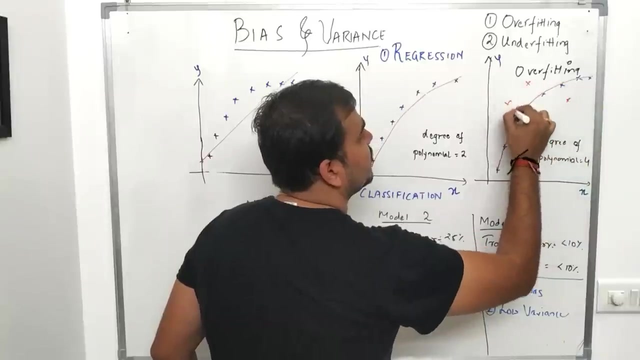 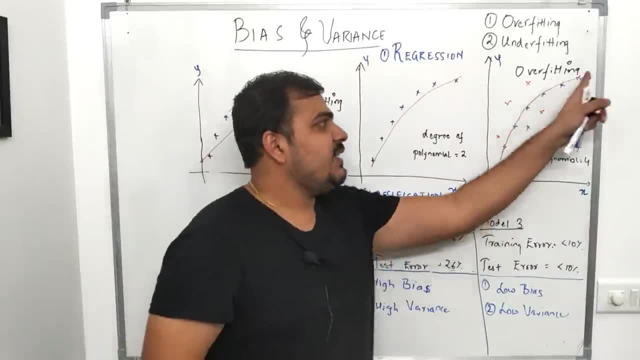 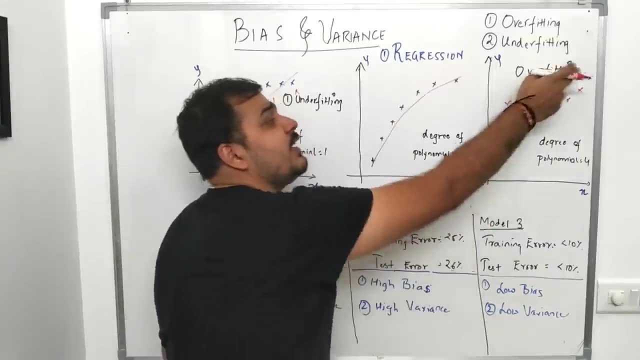 Right Now, just understand: will this best fit line satisfy properly? on the test data, Again, the error rate will be high In overfitting condition, even though for the training data the accuracy is quite high, But for the test data the accuracy goes down. 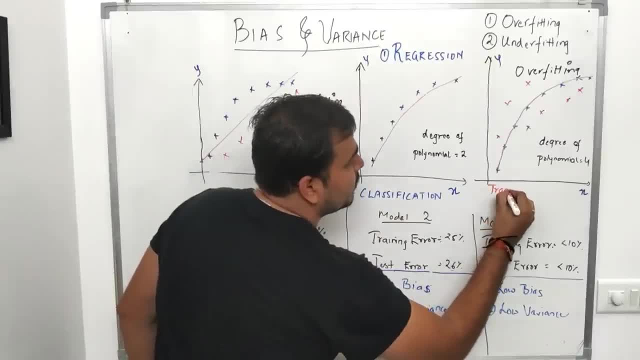 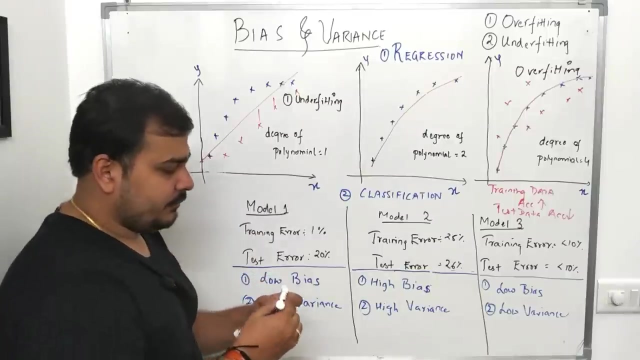 OK, So what, what I'm saying for the training data? for the training data, I can write it as accuracy is very, very high, But for the test data, the accuracy is very, very it's going down In this scenario. what is happening In this scenario? what is happening In this scenario? my accuracy of the 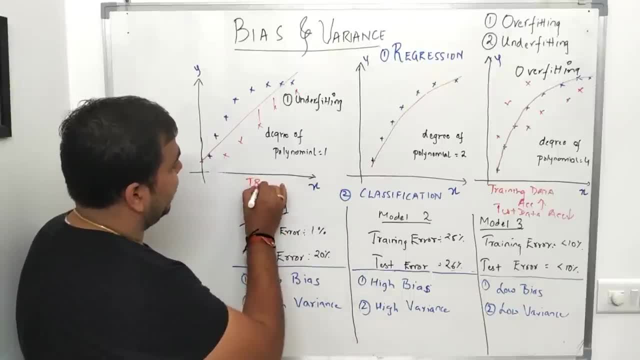 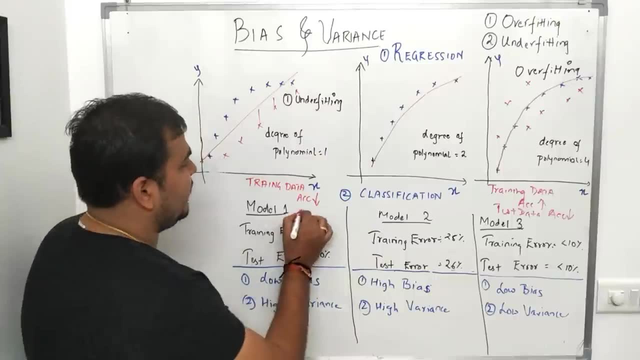 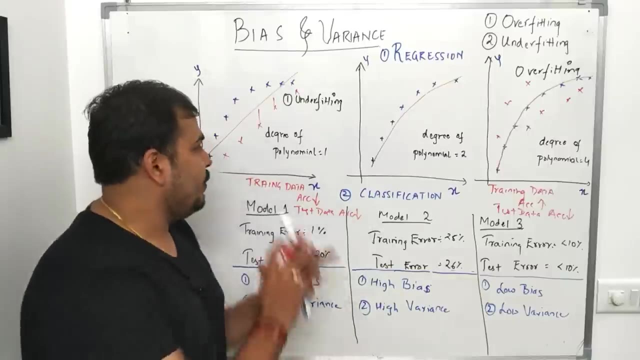 training data. My accuracy of the training data Accuracy is going down Right. For the test data also, the accuracy is going down Right, Right. I hope you have understood this. In this case, the training data, the accuracy is very high. 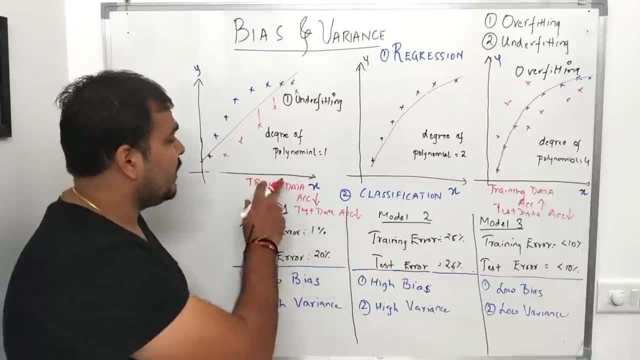 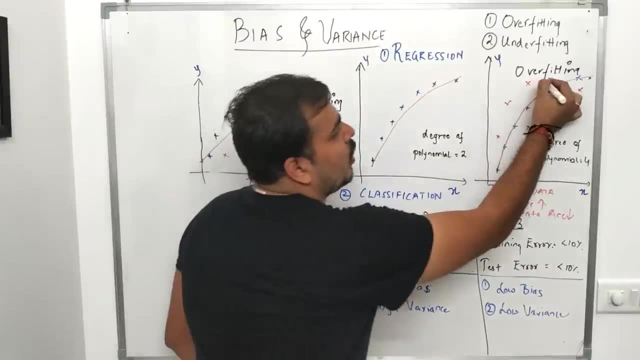 But for the test data the accuracy is very low. Vice versa over here. for the training data also, the accuracy is less, and for the test data also accuracy is less. So that scenario we call it as underfitting, This scenario we call it as overfitting. Our main aim should be in such that: 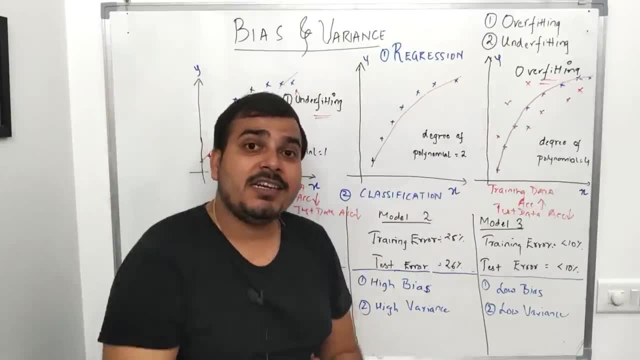 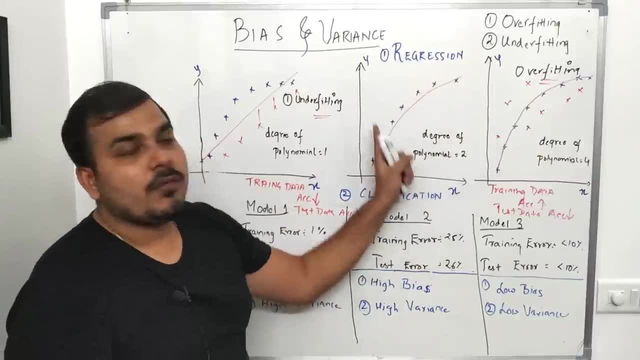 for the training data also, my accuracy should be high. and for the test data or for the new data also, my accuracy should be high. and that is actually solved by this particular degree of polynomial is equal to 2.. Now, in this scenario, out of these three models, you know I should 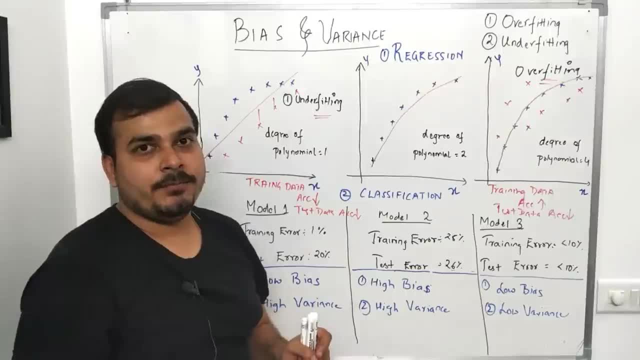 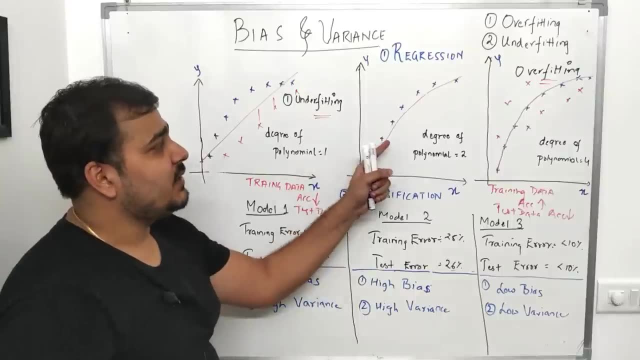 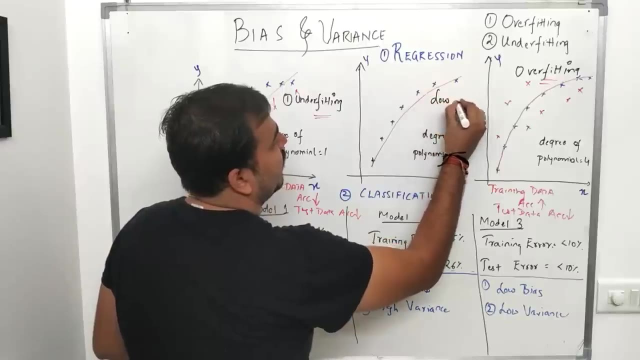 be selecting this model in order to solve my problem statement: Now, this is the most suitable model that we should select And in this particular model- you can understand, guys, this particular model is, You can say it- as this particular model is basically giving us low bias, low variance. 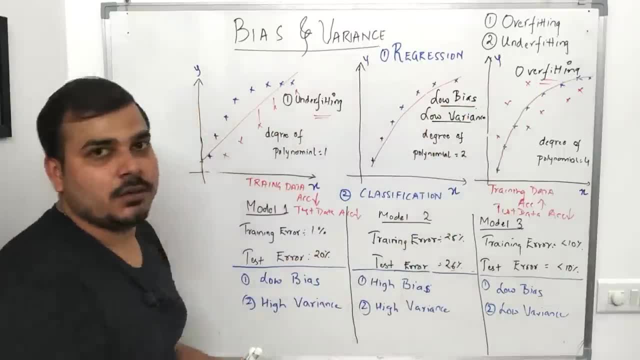 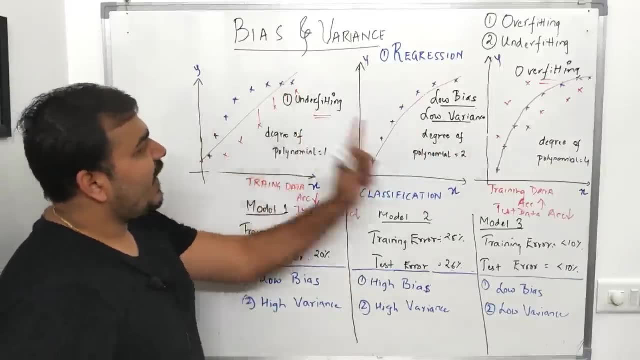 Low bias and low variance. Now let's discuss about this. What is bias and variance? I've just told you about overfitting and underfitting, But what about bias and variance? Now let's go over here In an underfitting scenario. in an underfitting scenario, I basically have 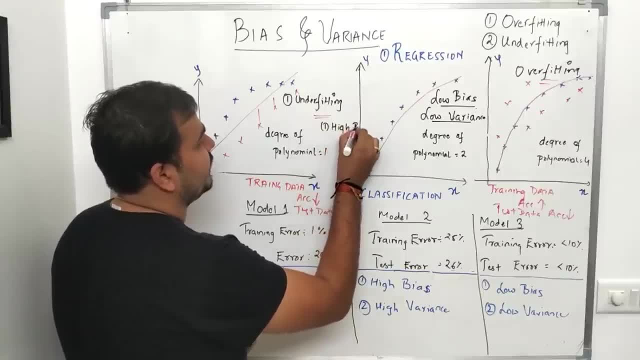 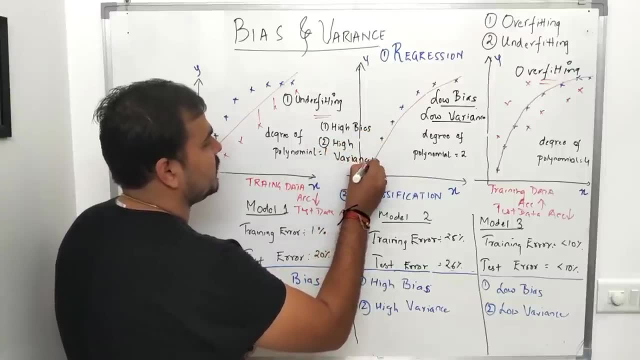 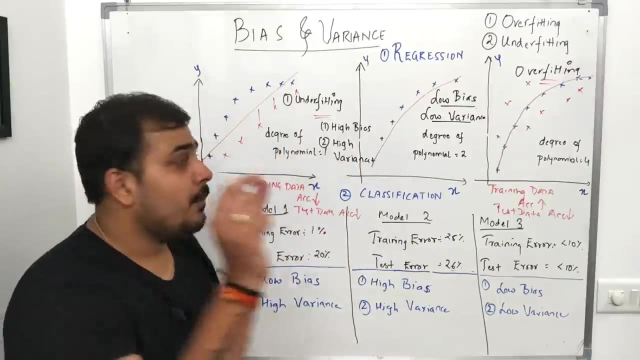 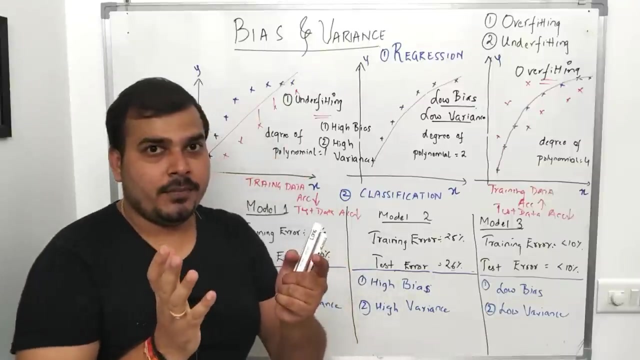 I basically have high bias And high variance. Always remember these things, guys. For an underfitting, I always have high bias and high variance. Bias basically means the error of the training data. Just consider, think in this particular way: OK, The error of the training data. Variance basically says: 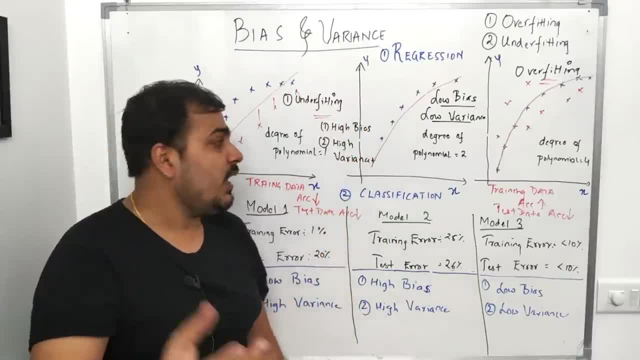 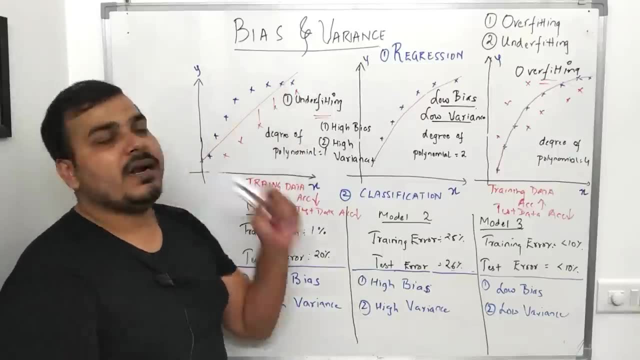 that it is the error of the test data. OK, So we have high bias and high variance. Now let's go back to the overfitting. So obviously, for the training data, the error is high. for the test data, error is high. That is what is the underfitting condition. Now let's go. 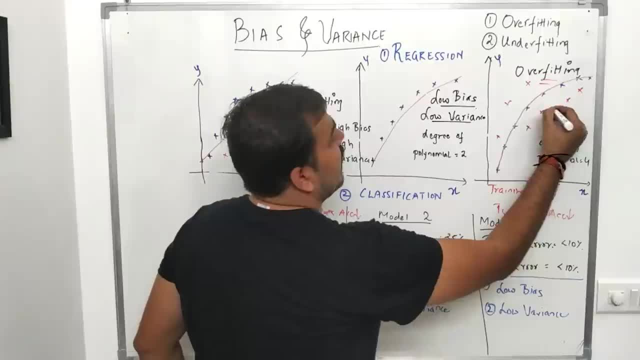 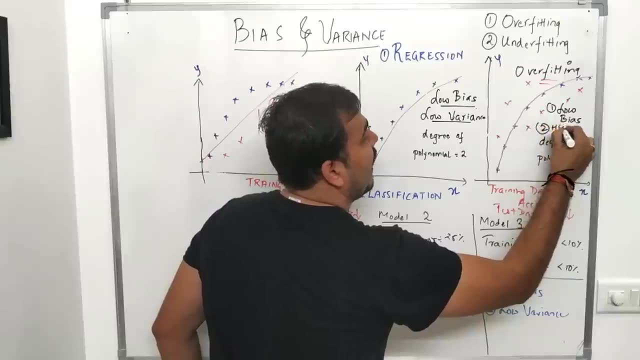 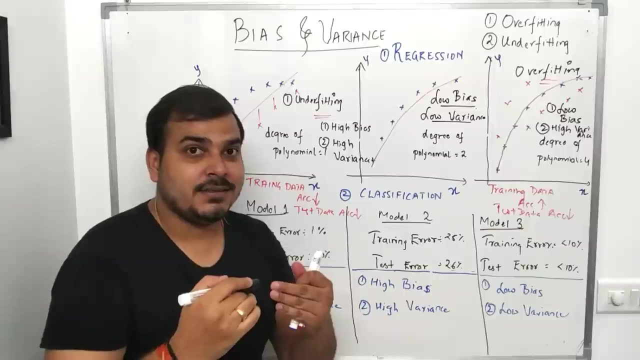 back to the overfitting In this scenario. I will be saying that over here I have low bias and high variance. Why low bias? Understand: for the training data the error is less Right. When the for the training data the error is less, We basically denote it as bias, Since 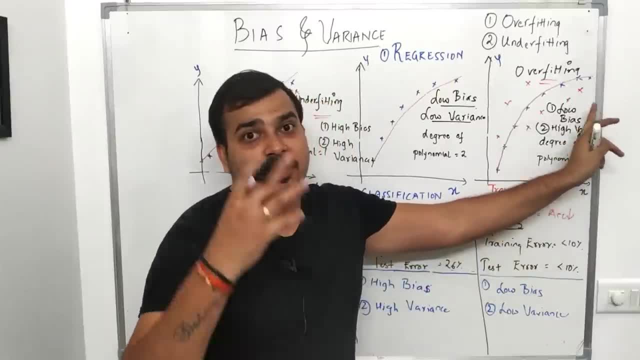 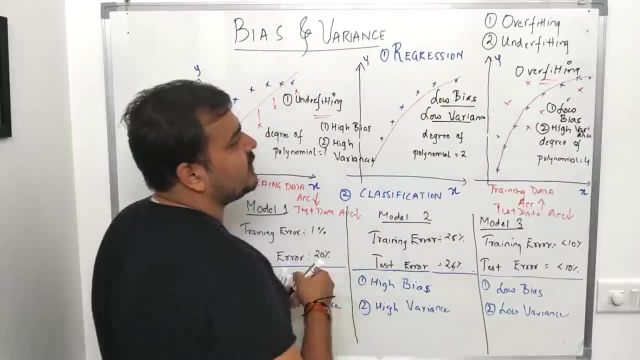 the error is less, we call it as low bias. But for the test data we are getting a huge error, so we are calling it as high variance. OK, I hope you have understood. So for this particular scenario we will be having low bias and low variance because for the training 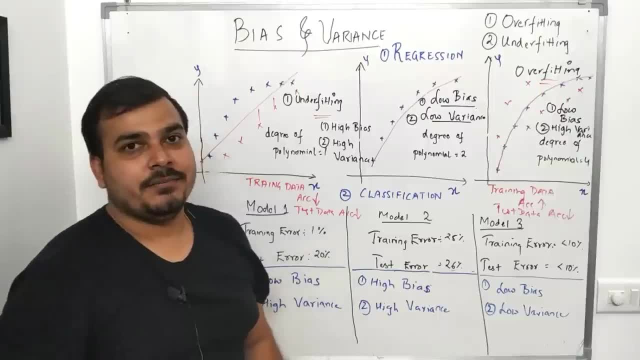 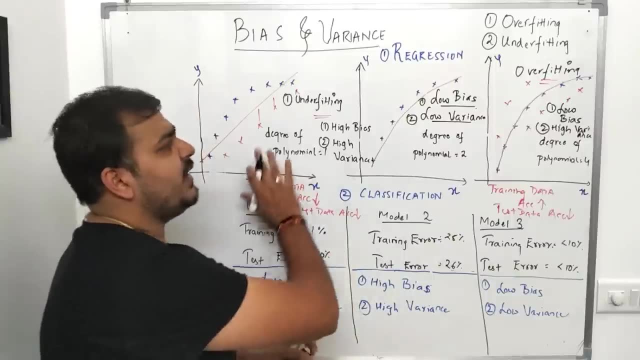 data also, we are getting less error. For the test data also, we are getting less error. Pretty much simple. I hope you have understood this. I hope you have understood it much more perfectly. If you have not just rewind it guys, Just rewind the video and try to understand. 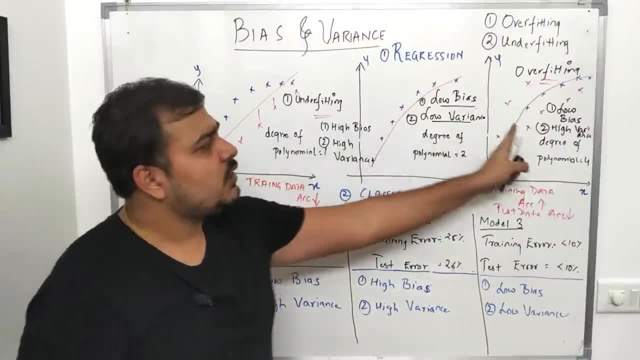 In this also for the new test data also, I will be getting low bias. But for the test data also, I will be getting high error. For this also I will be getting high error. Right When I compare this, this will be giving us a low error. OK, This was with respect to. 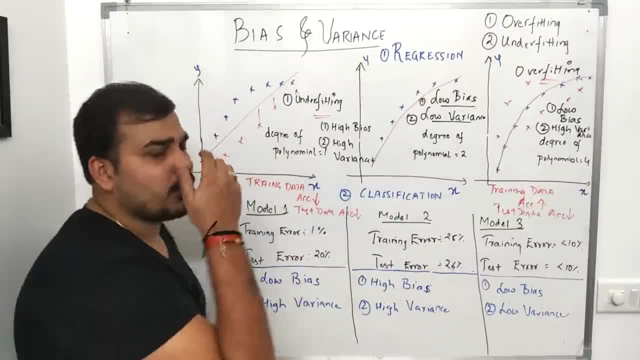 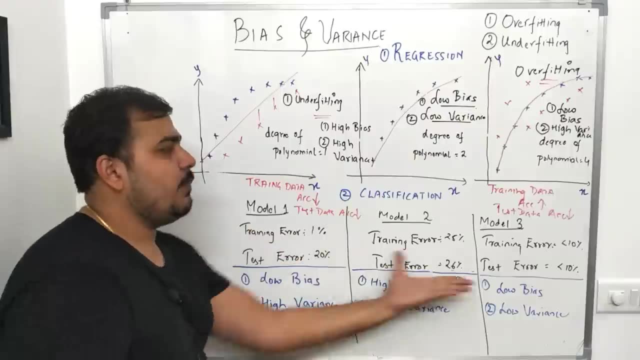 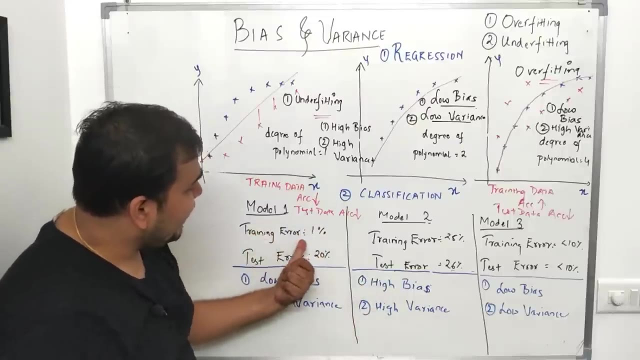 the regression problem statement. Now let us go to the classification problem statement. Now classification problem statement. Suppose I have used three models with three hyper parameter tuning techniques. I have done some hyper parameter optimization For the first time. my model 1. my training error was 1 percent. OK, Classification problem statement basically. 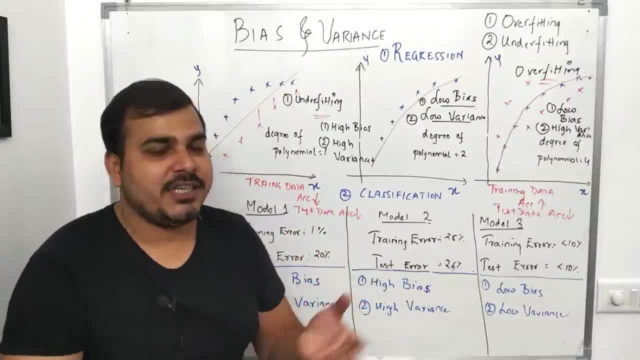 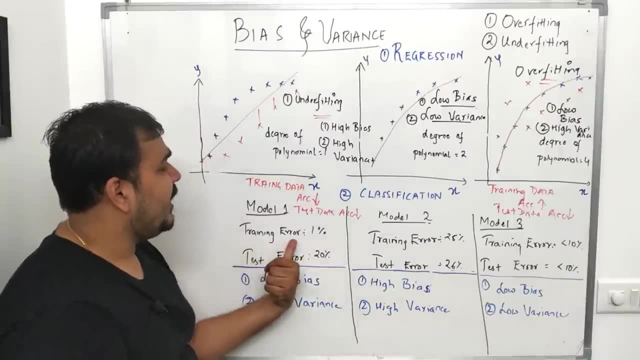 I am trying to compare whether my model is able to do a binary classification like yes or no, And usually you know that we use a confusion matrix for that Right. So over here. suppose my model 1 gives a training error of 1 percent. My model, model 1, gives a test. 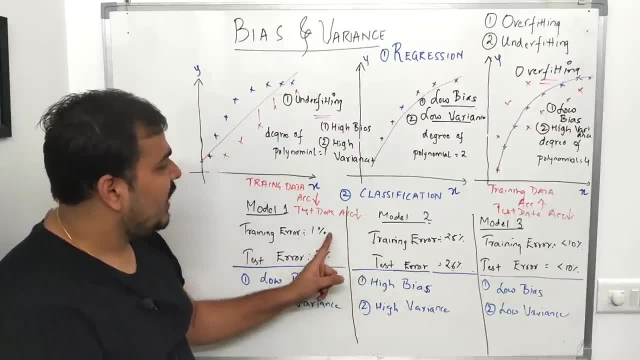 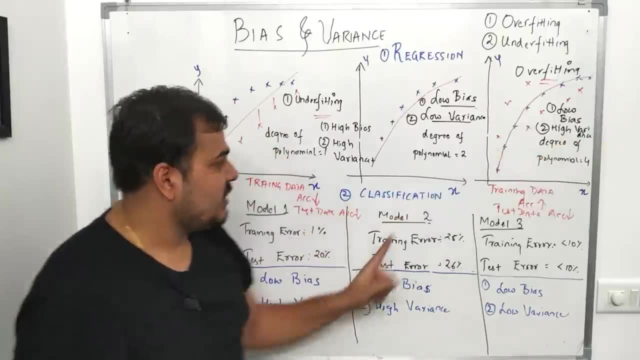 error of 20 percent. Now just understand what kind of scenario this is. 1 percent basically means low bias. Right Test error is high, So it will become high variance. So in this scenario, what is the scenario where? low bias and high variance? If we have low bias and 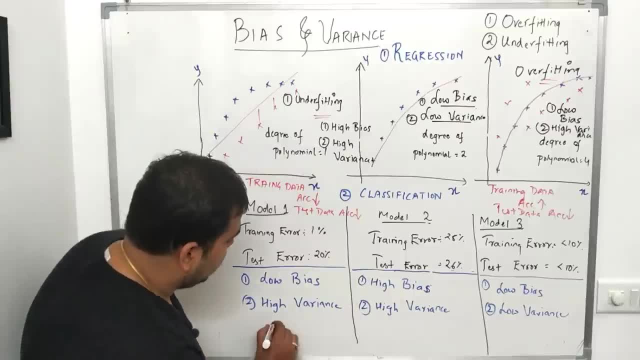 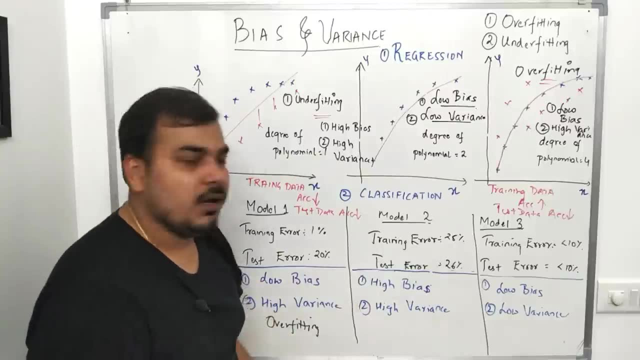 high variance. what is the scenario? This scenario is basically called as overfitting. This scenario is basically called as overfitting. Right Now, let us go to the second model. In the second model, my training error is 25 percent. My test error is 26 percent. Now, 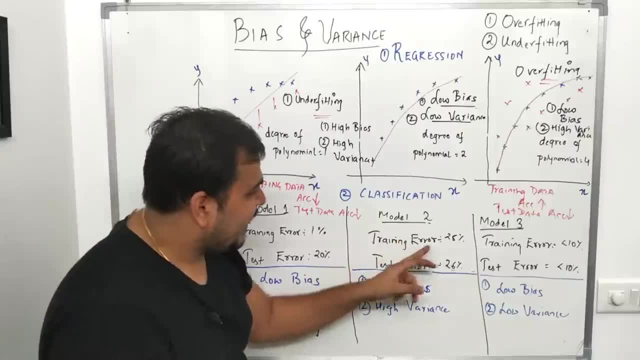 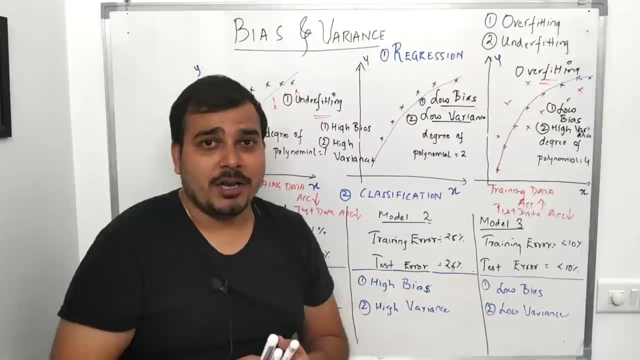 in this scenario, what do you think should be? You know, training error is given 25 percent. Again, understand, guys, if your model is just 75 percent accurate, I think you should try to improve that particular model. Yeah, So it also depends on the domain that you are. 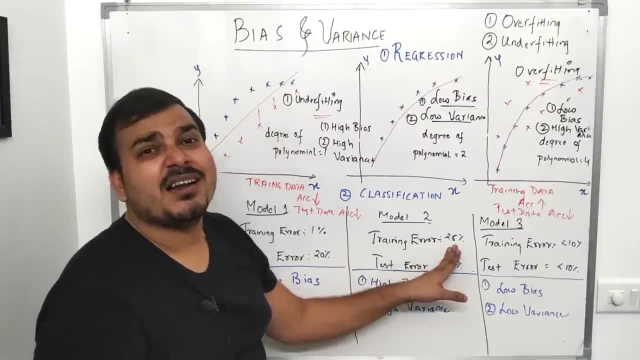 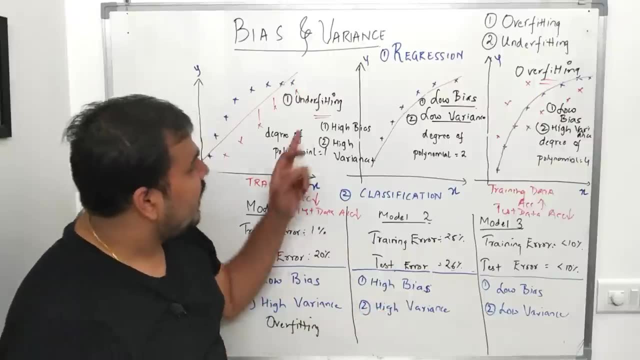 working, But right now I'm considering that this is actually a underfitting problem. What is underfitting problem? High bias, high variance. Since my training error is high, I'll say it as high bias. If, since my test error is very high, I'm going to say it as high variance. 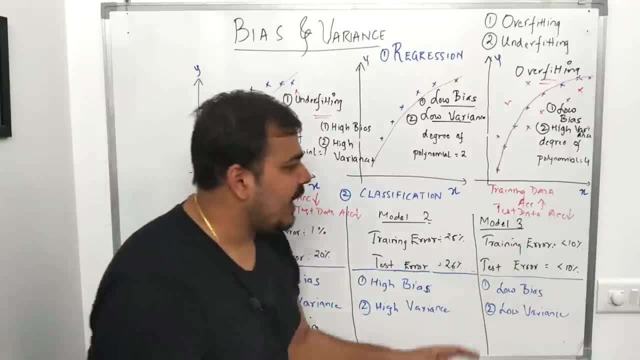 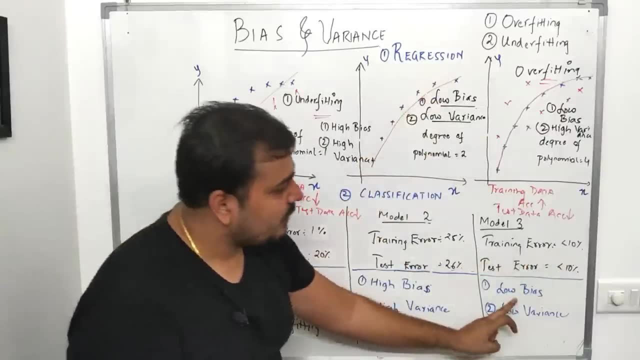 OK, Now next thing is model 3.. In model 3, what is happening? My training error is less than 10 percent. My test error is less than 10 percent. Now, this is the scenario that we are covering over here, which is nothing but low bias and low variance. So this becomes: 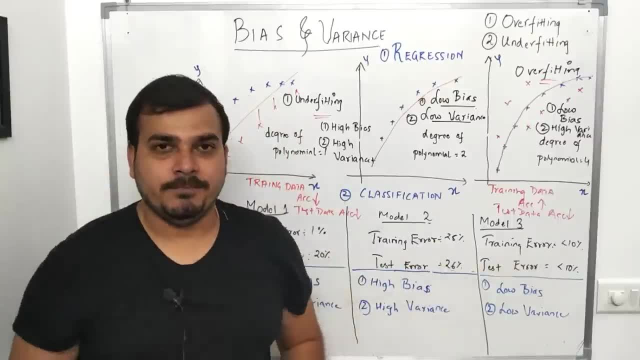 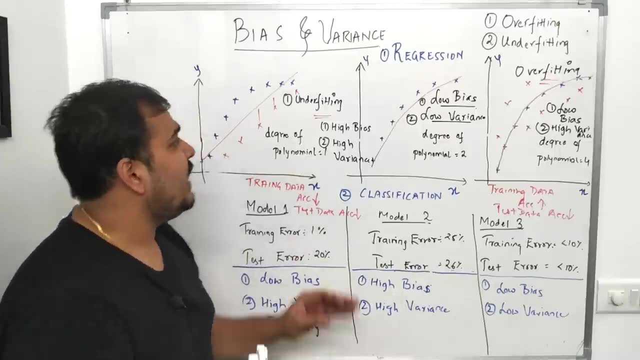 an underfitting problem, This becomes the most difficult Generalized model, Right. So I hope you have understood these things Now. this is pretty much important to understand what I'm going to do. guys, I'm just going to rub this diagram. 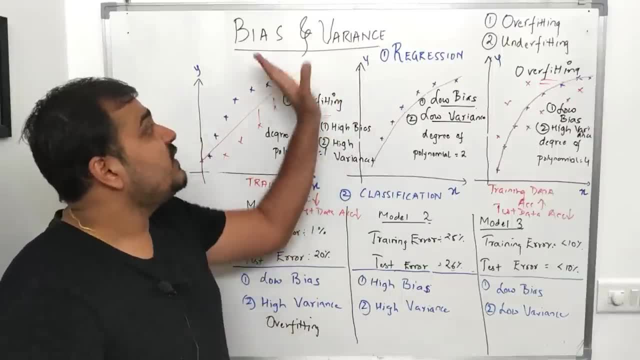 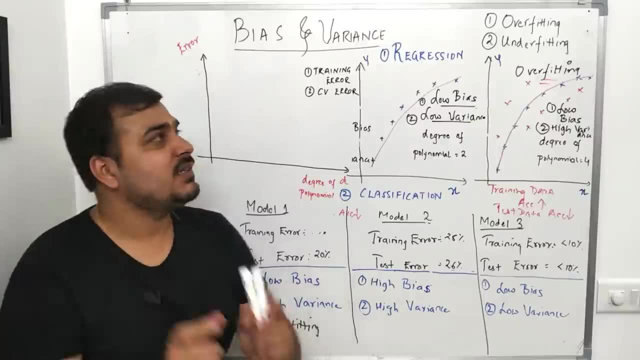 OK, and I'm going to show you a general representation of this bias and variance, how it is shown in graphical order. OK, we'll try to understand that. OK, guys, let us go ahead and try to understand the general representation of bias and variance. I'll take the same example, what I had actually 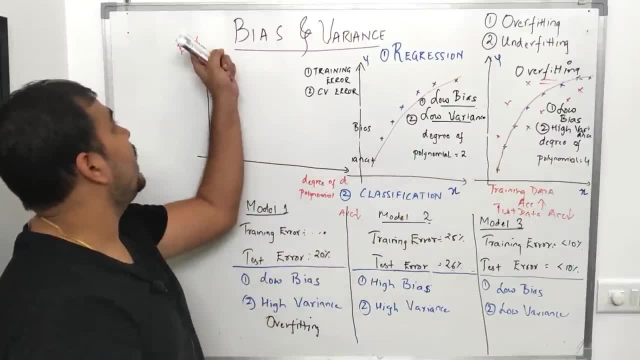 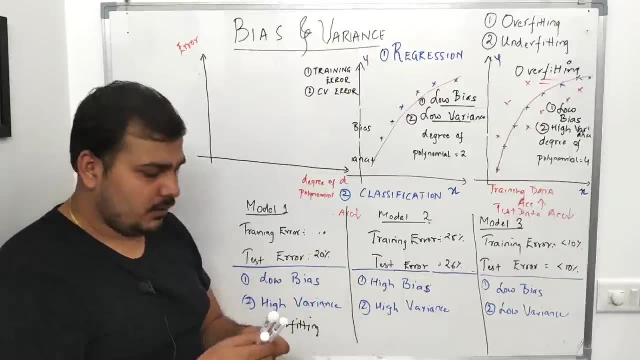 taken over here in my X axis is degree of polynomial. Over here In my Y axis it is error. So understand, if you have an underfitting condition what will happen. Usually the error rate will be high, So error rate for the training data will also. 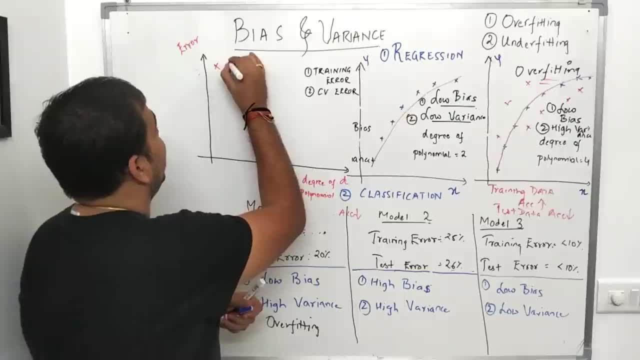 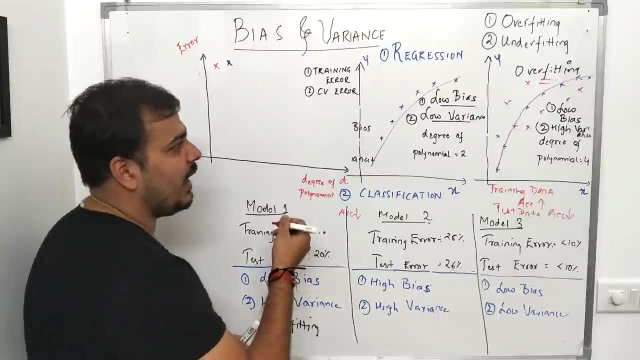 be high, Error rate for the test data will also be high, Right, OK, Now let us go and try to understand this overfitting condition In the overfitting condition. what will happen In the overfitting condition? if I take this particular example over here, or let me just 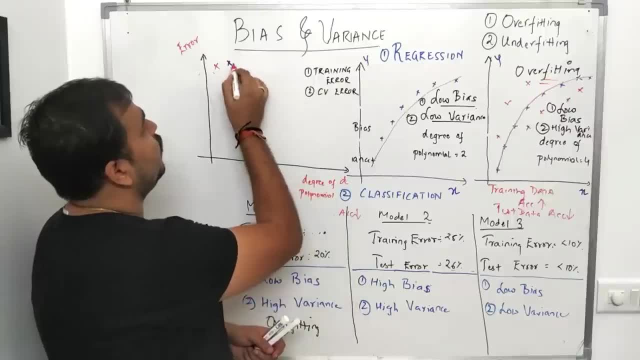 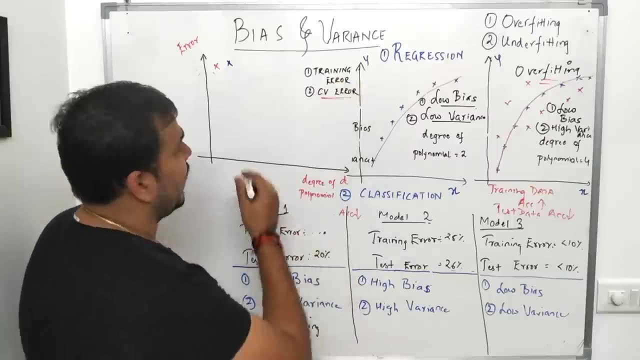 OK, understand, guys. This red point is basically my training error. This blue point is basically my cross validation error, or you can also say it is test error. OK, So we'll just try to write in this particular way. OK, Now for the overfitting condition. 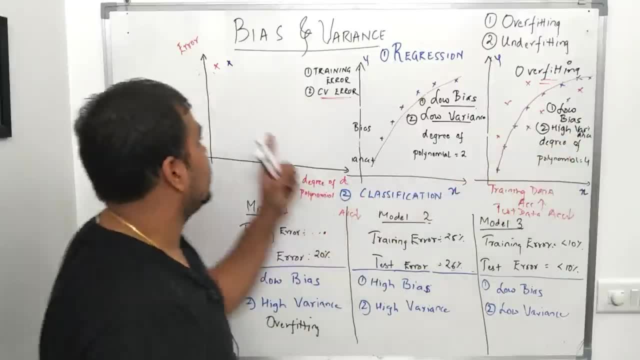 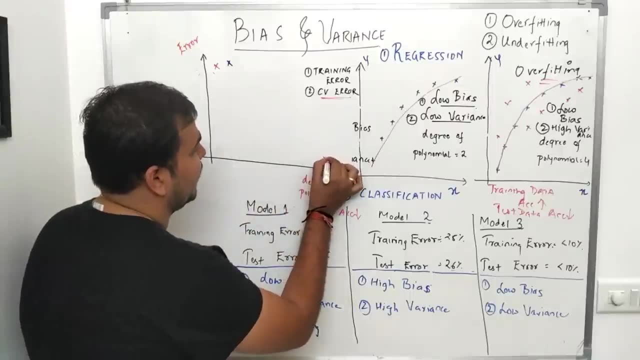 you can. you know that I have low bias and high variance. So my training error, for the training data- I mean for the training data- it will become less. So suppose I am going to mention this particular point. OK, Now, with respect to this particular point, you 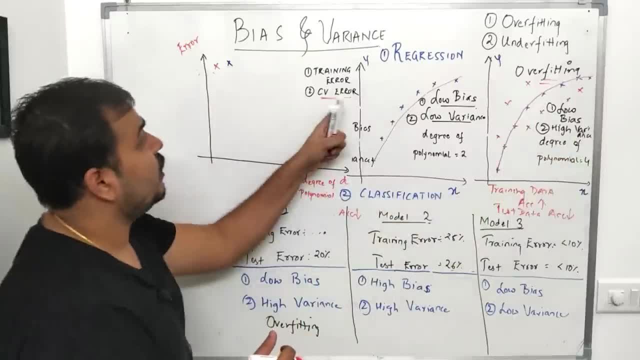 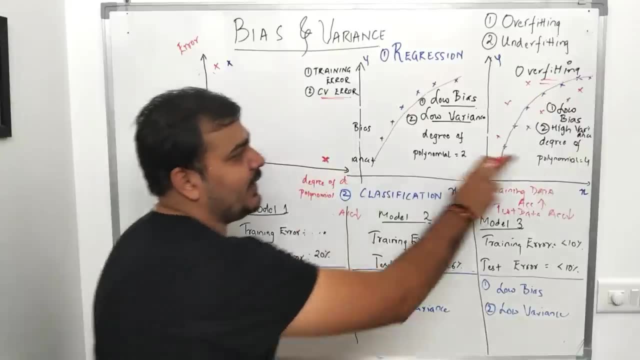 you can see that for the test data it is high variance, So the error rate for the cross validation error will be high. be high in the case of overfitting problem statement right when my degree of the polynomial is high. in this case, my degree of polynomial is high, so I am just going to keep this particular. 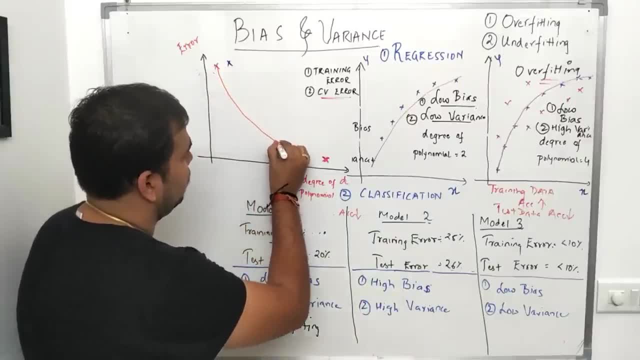 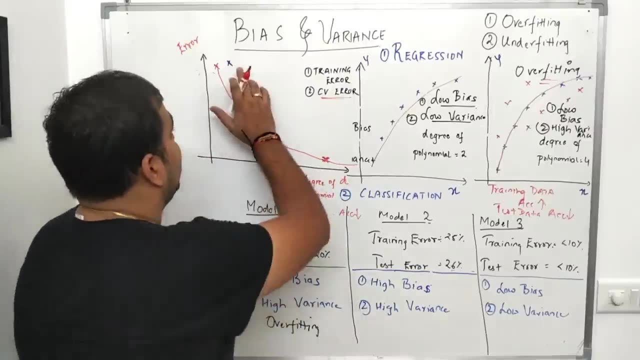 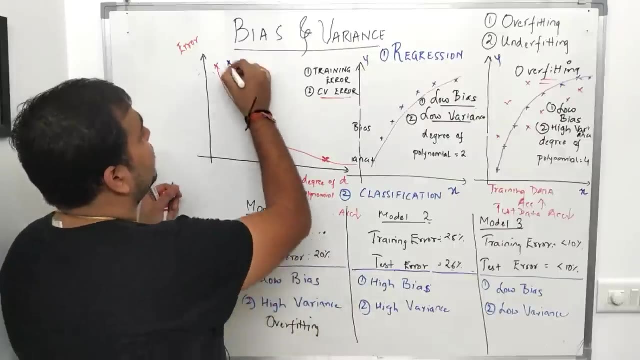 point like this. let me combine this particular point like this: okay, so I have combined this particular training error like this. it will go like this itself: okay, fine, now about this particular point. okay, you will be able to see that. you will be also able to see that. 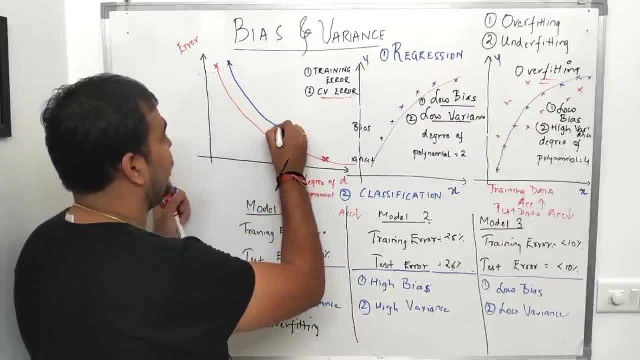 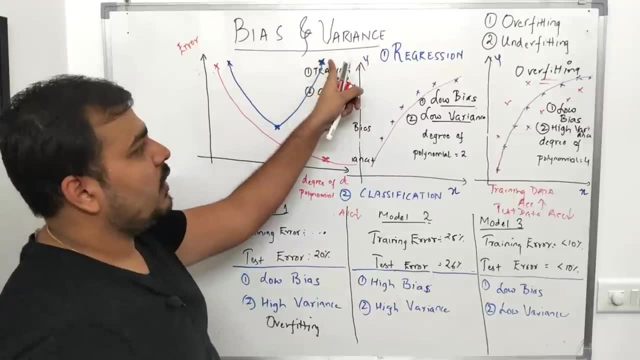 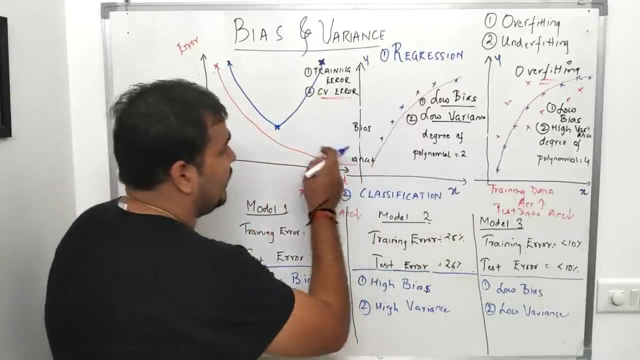 this points will also reduce, like this, at certain point, and then after that it will again increase. okay, now, this particular point that I was talking about, it is nothing but high variance for the same degree. okay, high variance for the same degree, because I told you, oh, till at certain point again, your cross validation error will be reducing, but after 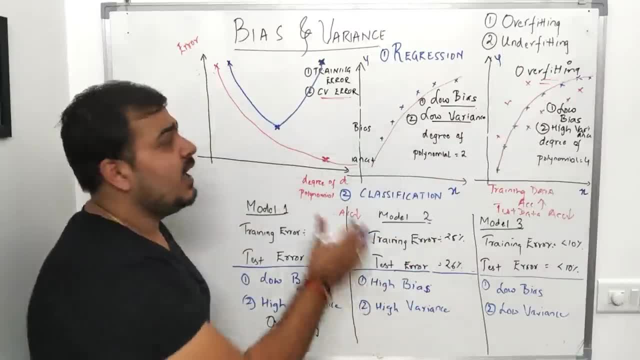 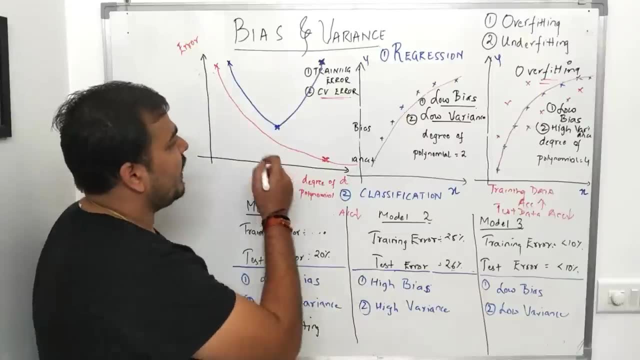 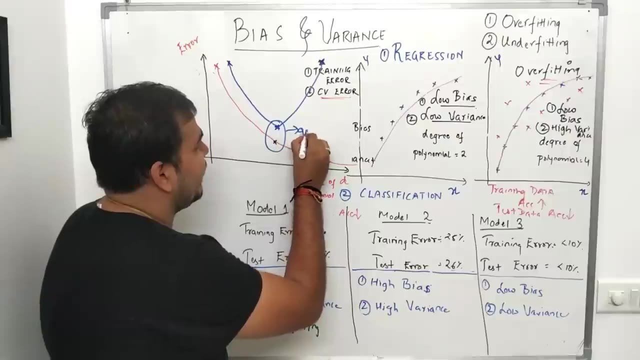 certain point, you know, since you are overfitting the problem statement. it's the accuracy- sorry, the accuracy or the error rate. The error rate will actually be increasing. so our aim is to actually find out a model. you know where this generalized formation can come. this generalized model can be created. 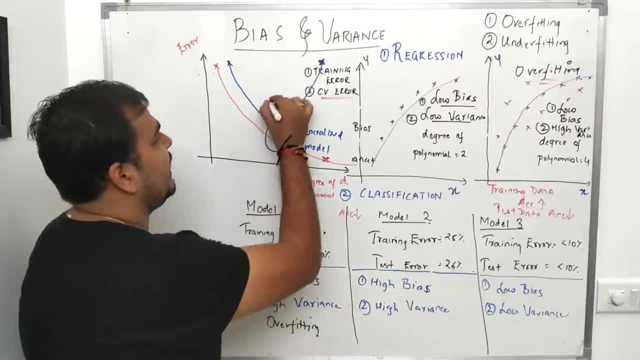 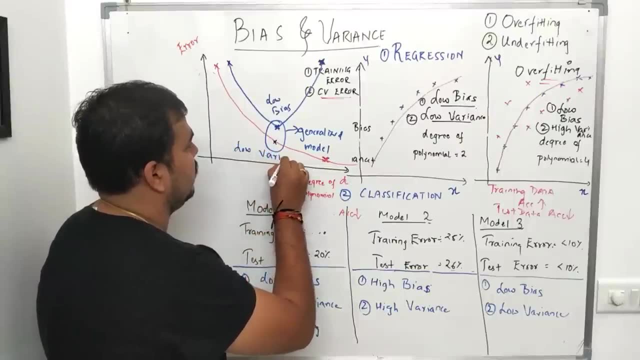 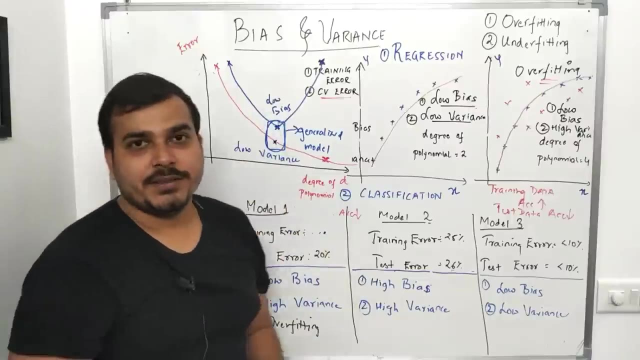 like, based on the errors that we are getting over here, and this scenario is nothing but low bias and low variance. Now, in from this particular graph, you can see that this particular point is actually having low bias and low variance. pretty simple, guys. so I hope you have understood this is. 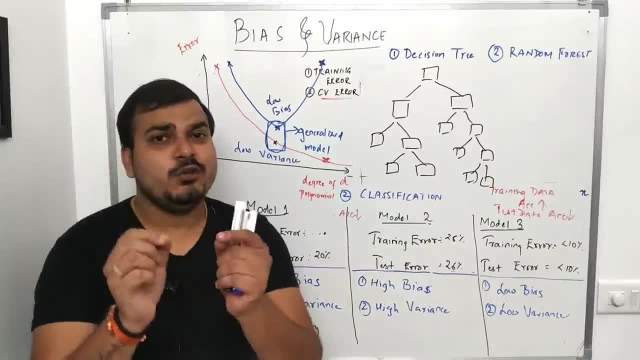 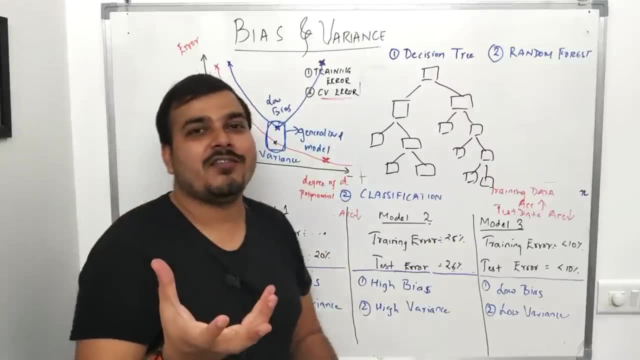 the general representation of bias and variance. let us go ahead and take some examples with respect to decision tree and random forest, and then we will try to understand whether it is an overfitting condition or underfitting condition. now, by default, you know that, guys, decision tree creates disguised of trees itself right completely to its depth. it takes all. 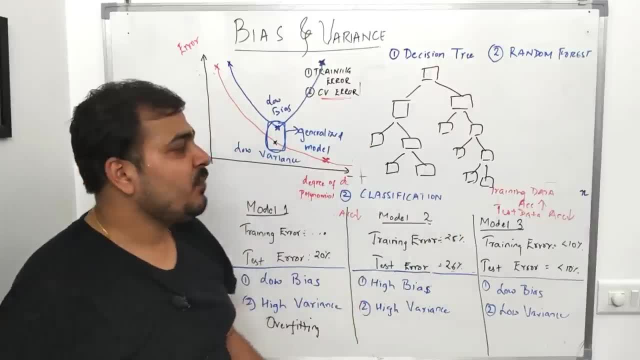 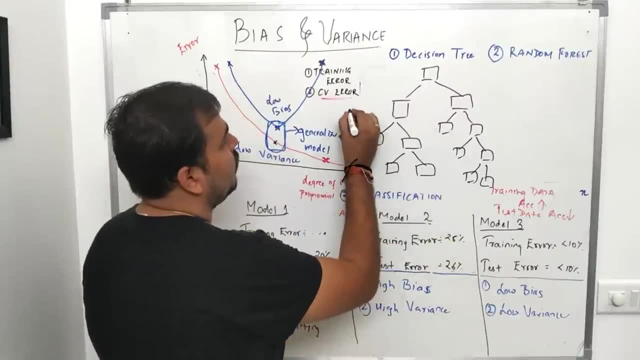 the features and then it starts splitting to its complete depth. okay, now, when it does this, This scenario is just like an overfitting condition. okay, this scenario is just like an overfitting condition. now, in overfitting, you just split all the decision tree till. 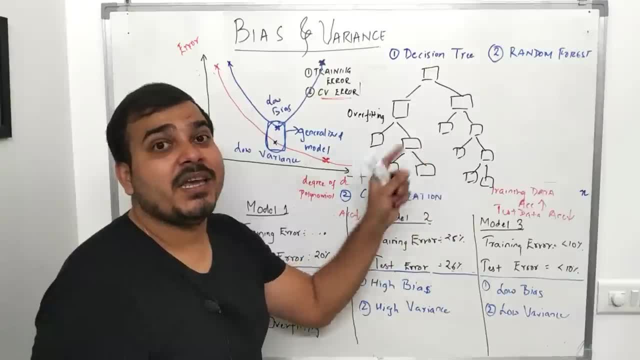 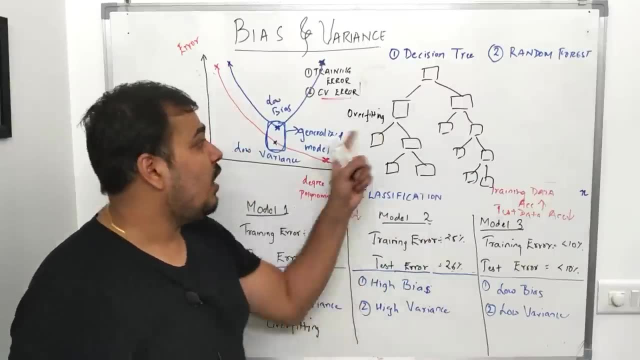 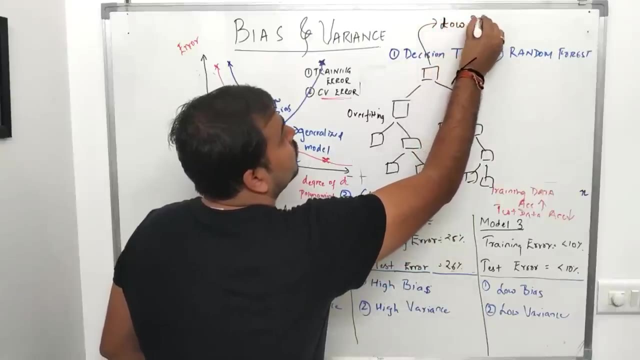 its complete depth. definitely, for the training data, this may give you a very good result. okay, the error rate will be less. but for the test data guys, this scenario will not work. now, this scenario, this decision tree, basically has a scenario of, you know, low bias, low bias. 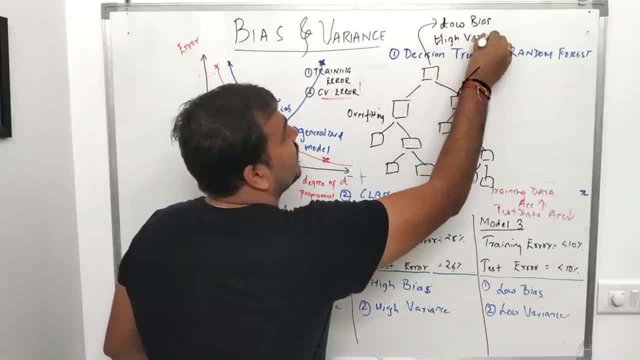 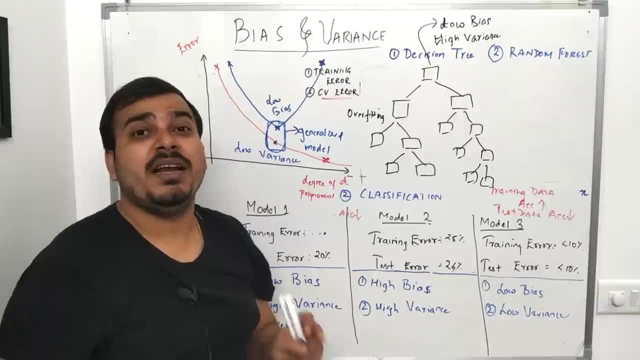 and high variance. It has a scenario of low bias and high variance because, understand, because we are just training on the data, on the training data itself, and we have splitted it to its complete depth. you know, for the test data, definitely this is not going to give a very good result. you. 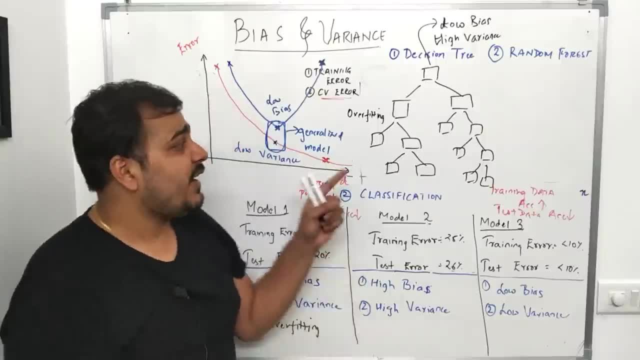 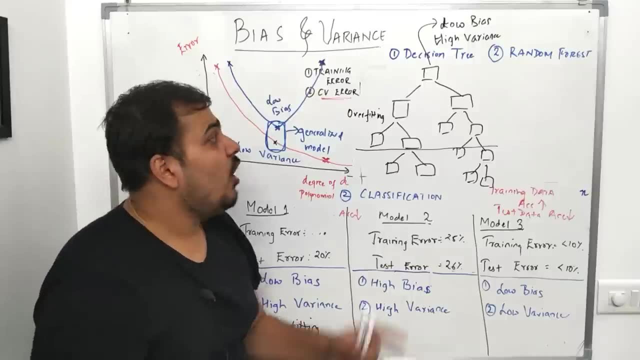 know. so because of this we use techniques like decision pruning. we try to only create the decision tree up till some depth. you know, after that depth will not still split. so that is the way of actually converting this high variance into low variance. and again, there are lot of hyperparameters. 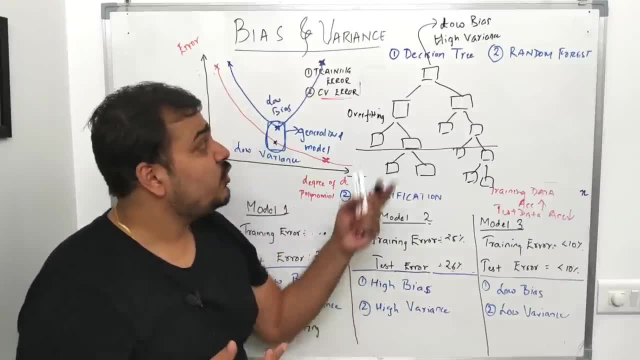 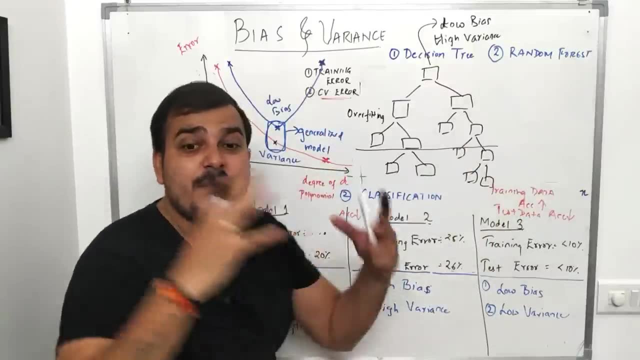 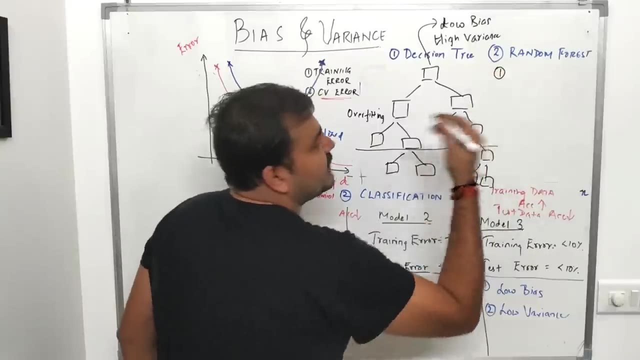 There are lot of techniques- hyperparameter tuning techniques, guys- and definitely should go and explore about decision tree. regarding that, now let us go ahead and take an example of random forest. in random forest, we use multiple decision tree in parallel. okay, multiple decision tree in parallel. and when we consider random forest, guys, when we consider random forest, 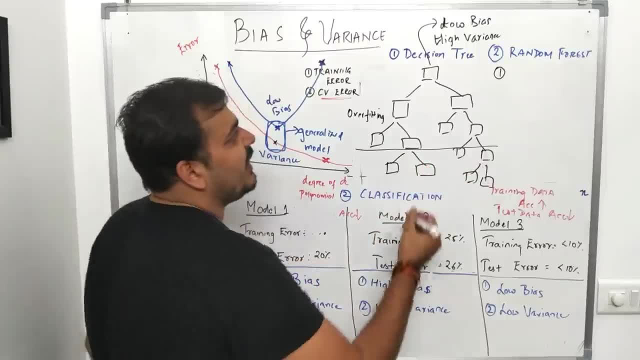 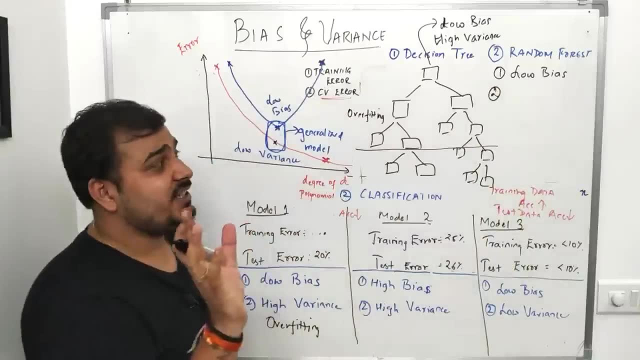 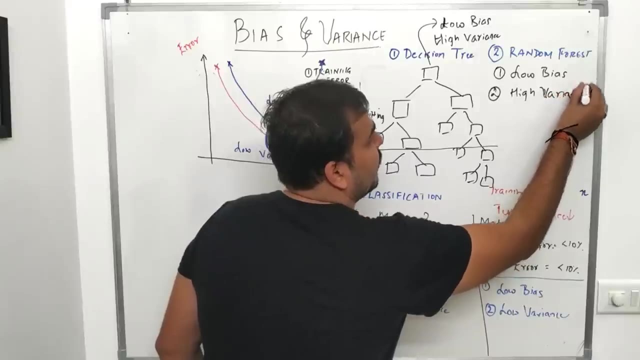 since we are using multiple decision tree in parallel, we basically have a scenario of something like low bias. and since we are, since we are using decision tree again, I am telling you, initially it will have this kind of property of high variance, low bias and high variance. this will be the property with respect to each and every decision tree. but since we 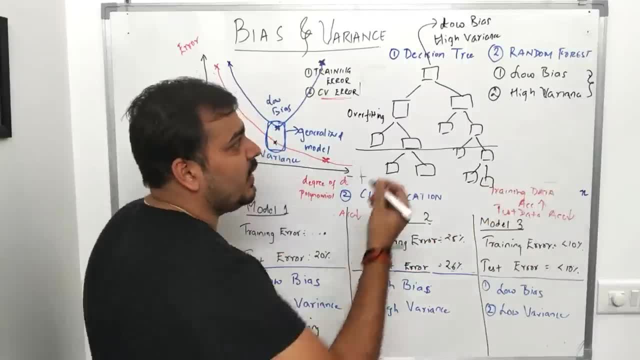 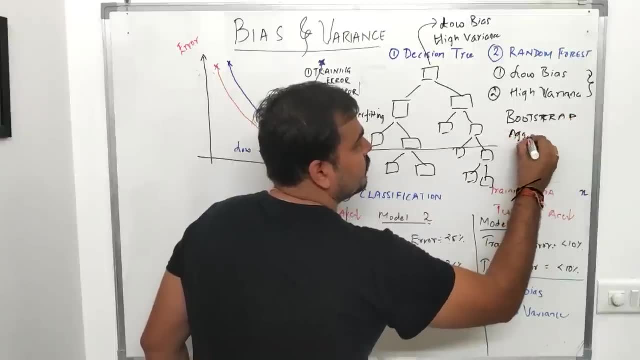 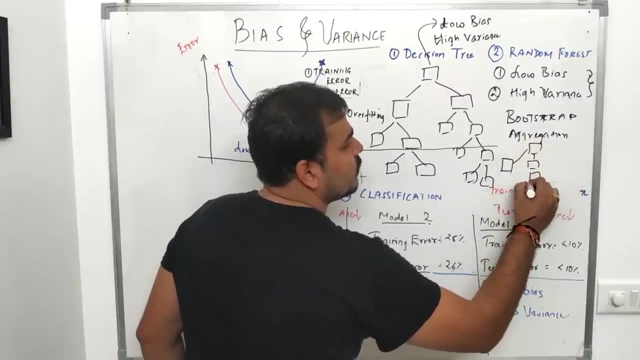 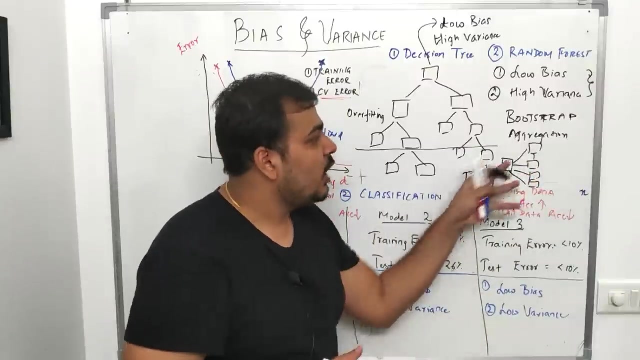 are combining those decision tree in parallel because, understanding random forest, what is that? it is basically called as bootstrap aggregation. bootstrap aggregation in bootstrap aggregation. what we do? we take a data set, we give it to multiple models. okay, we give, we give this data set. We don't give the whole records, but we give a partial, some n number of records to different. 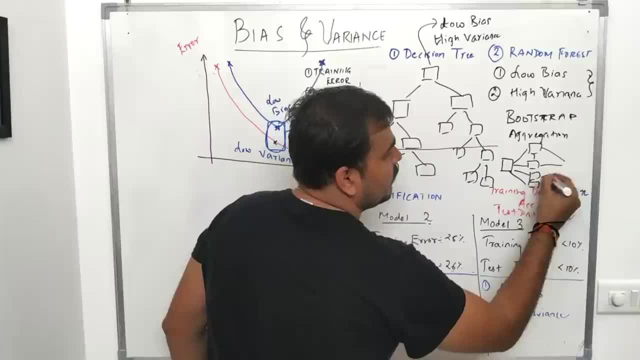 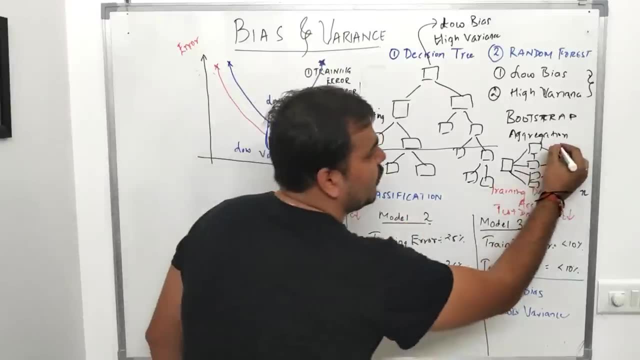 different decision trees, okay, and finally we get the output and we aggregate it. we aggregate it and then we see that who suppose many models are actually given a value as one? then we will consider that the output is one. if many model gives us the output as zero, we will. 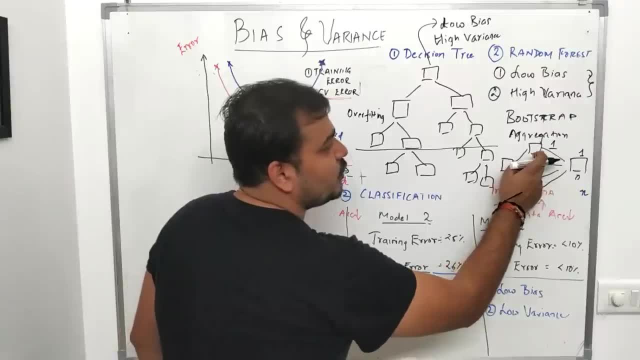 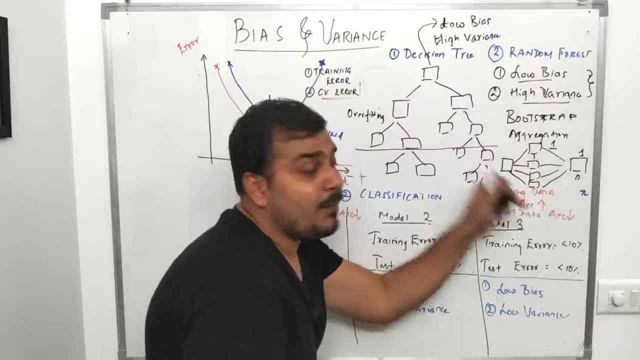 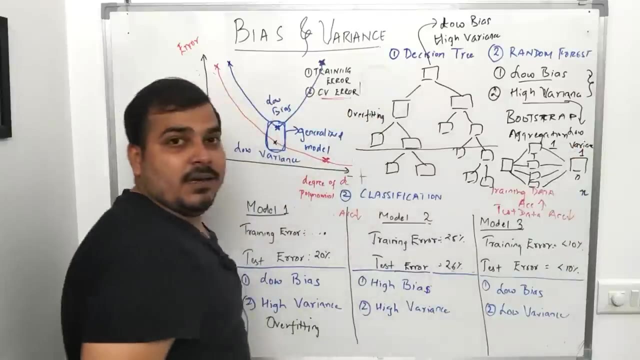 consider the output as zero now, initially, since I was using many decision trees and each and every decision tree has a property of low bias and high variance. If I combine this in a parallel way, this high variance will get converted to low variance. okay, how it is getting converted to: from high variance to low variance, since we are using 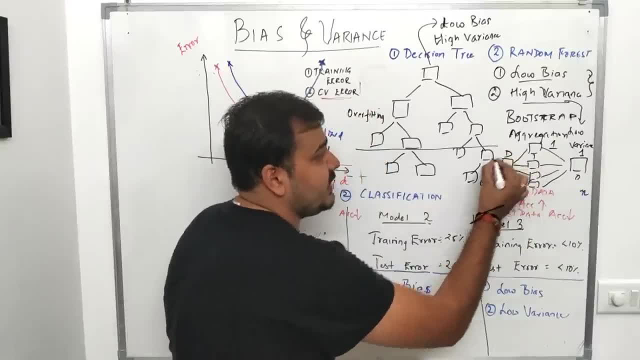 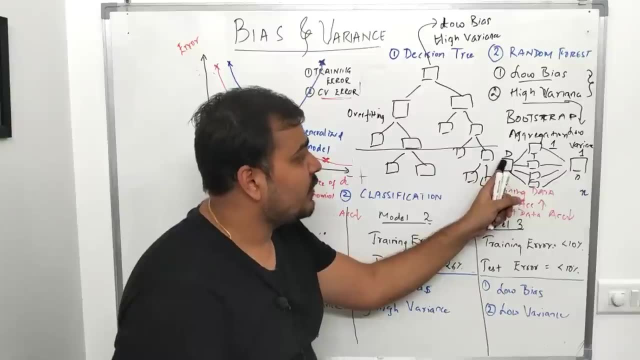 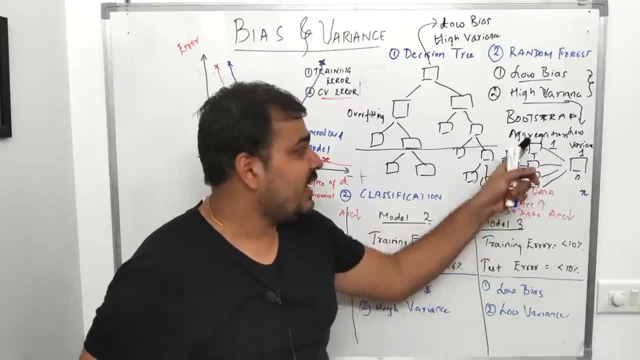 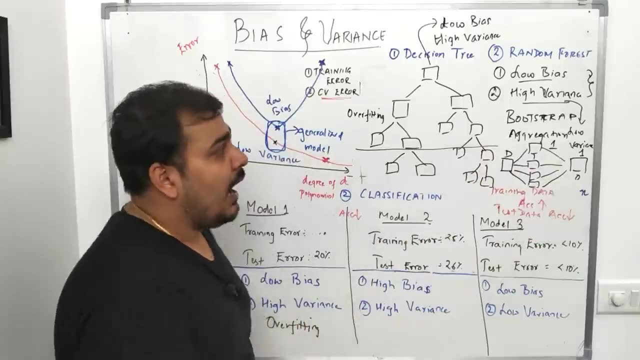